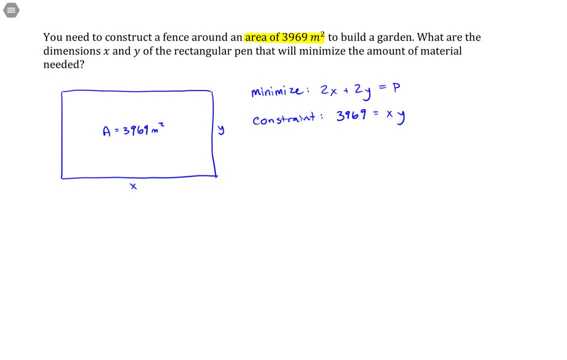 need to minimize for these two variables perimeter. then X and Y. We can't do anything with that until we get it down to just two variables. So that's where the constraint will come in. So I could solve the constraint for X perhaps and say X equals 39.69 over Y And then plug that into the perimeter. So the perimeter now would: 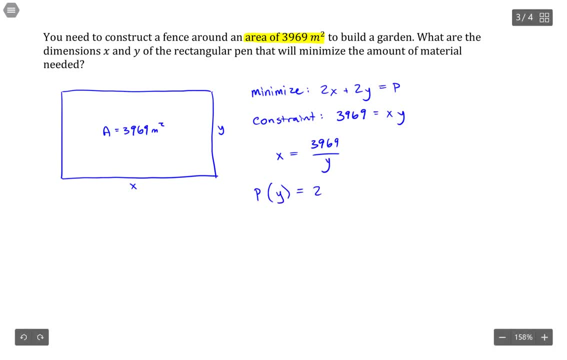 be entirely of the variable Y, and this would be two times X plus 2Y the cost. And then I could do the constraint 39, 69, divided by y plus 2 times y, Because all I've done is I've substituted in for the variable x. 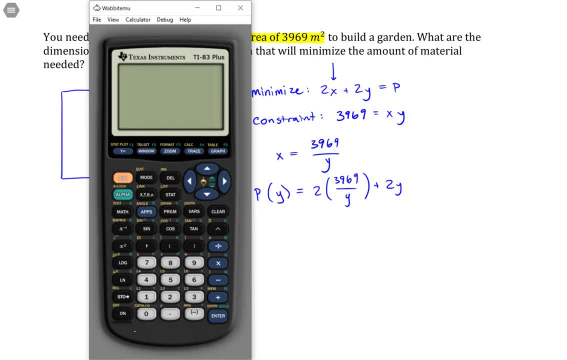 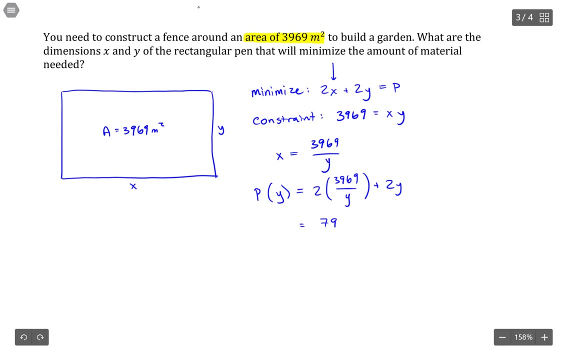 So let's simplify here and we'll say: 2 times 39, 69 is 79, 38.. So this is 79, 38, divided by y plus 2y. Okay, now to minimize this, we need to find its derivative and set that derivative equal to 0.. 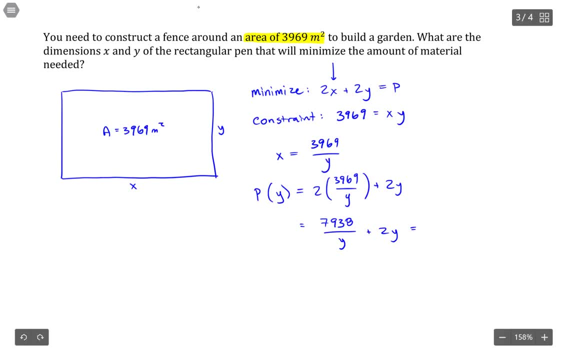 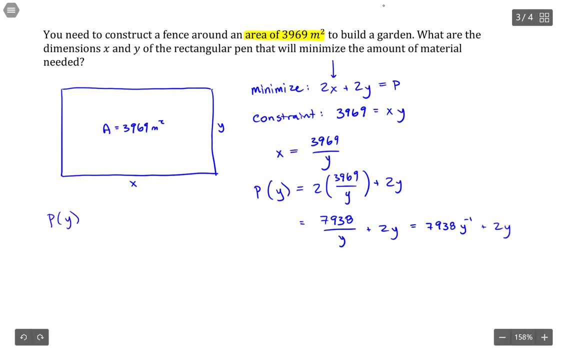 So the derivative of this function, since it's actually of the form 79,, 38, y, to the negative 1, plus 2y. Okay, now I'll just come over here And do that derivative. So that would be, let's see, bringing the negative 1 down times this constant. 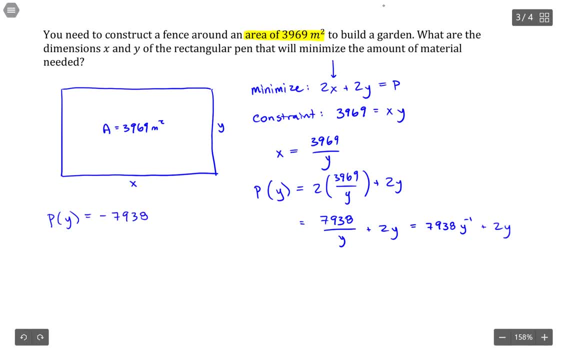 That would be negative 79,, 38, y to the negative 2nd power, because I subtract 1 from my exponent, Then plus 2y, its derivative is just 2.. Now I need to set this equal to 0.. 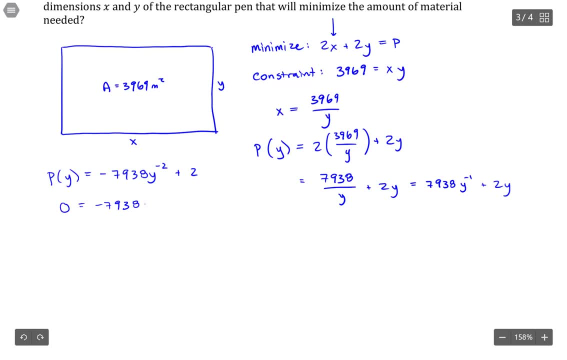 So 0 equals negative 7.. 79, 38, y to the negative, 2, plus 2.. And then solve. So let's see if I I'll just move this term over to make it positive- 79,, 38, y to the negative 2nd.